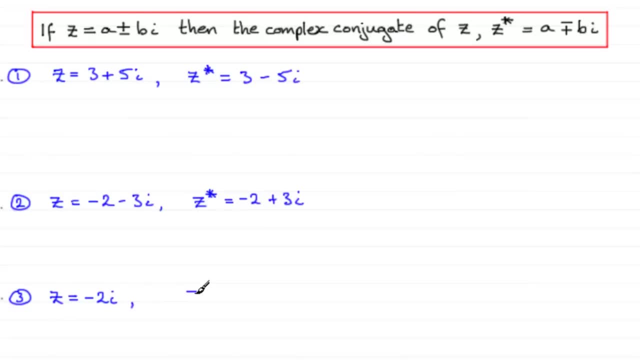 2i, then the complex conjugate of that z star would be 2i. When you've got a complex number and it's complex conjugate, we often call this a complex conjugate pair. So if you had thataton, thataton is equal to 2i, then thataton is equal to 2i. So this is. 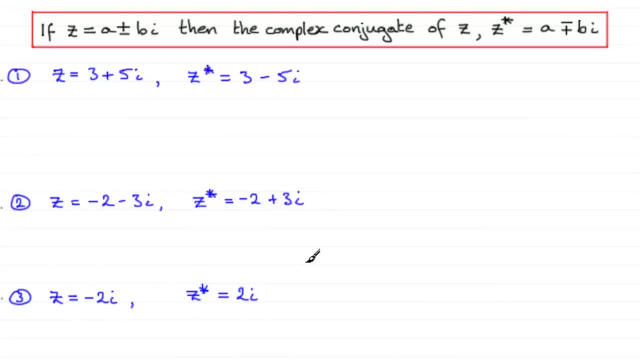 a complex conjugate, but that's true probably because of thequele same numbers applied to them. Now, when we have complex numbers and they're complex conjugate, two things happen that are very special that we can use later on, as you'll find out in later tutorials. 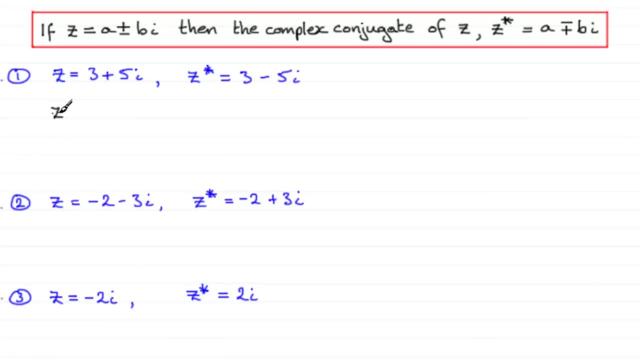 Conjugate components are complex numbers. Conjugate components are complex numbers. Conjugate molecules are complex numbers. Conjugateots have complex numbers. Conjugate equipments have complex numbers. Between them are four plus twoi, and that's what it is. Conjugate components hold the double Н, So it's just one to zero. and then we add two 硫 in neutral JavaScript. that what? When you look at that particular sentence, that's equal to 0% and that's only one number. 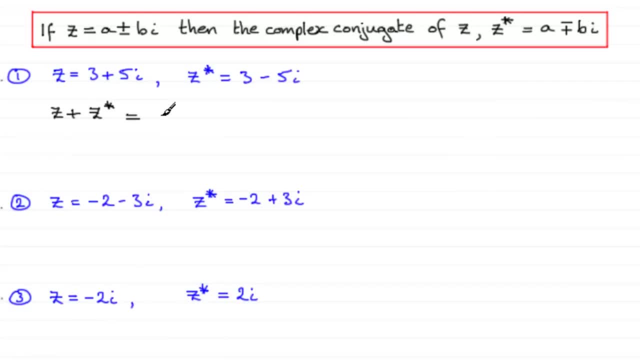 together, then we always get a real number. Look z plus z star. if we were to add these two together, 3 plus 5i plus 3 minus 5i, then what happens is the 5is cancel one another. 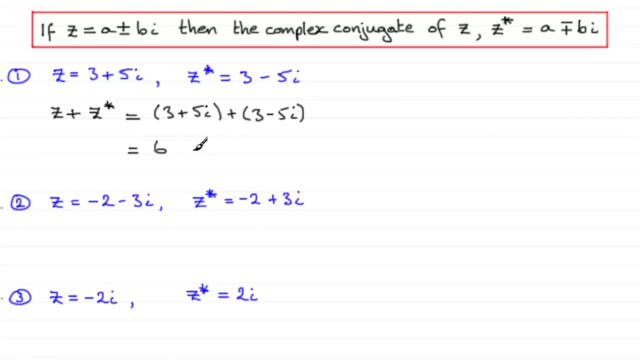 out and you've just got 3 plus 3, which is 6.. And if you were to multiply the two complex conjugate pairs together, z multiplied by the complex conjugate of z, we end up with doing 3 plus 5i, in this example, multiplied by 3 minus 5i. And if you expand this, you've 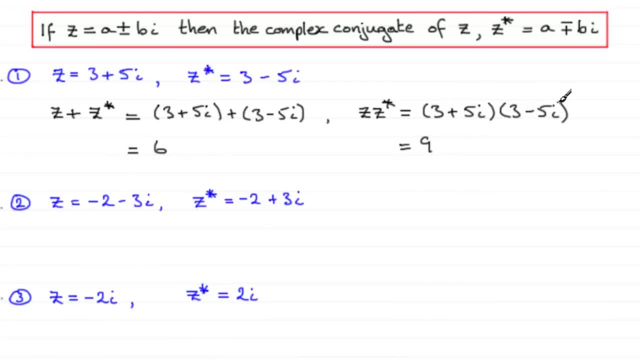 got 3 times 3,, which is 9, then you've got 3 times minus 5i, which is minus 15i, 5i times 3,, which is plus 15i, and plus 5i multiplied by 3.. 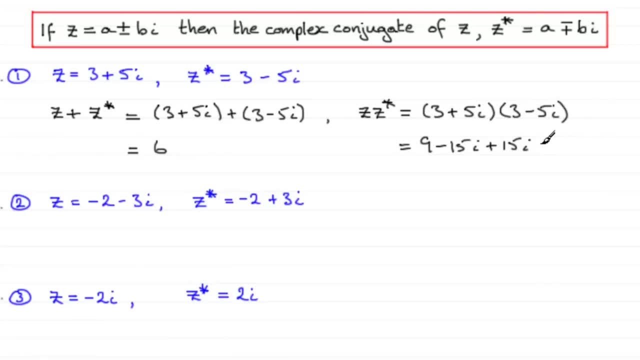 Multiply that by minus 5i, well, that's minus 25i squared, which is plus 25.. And what we end up with is that we get 9 plus 25, which is 34.. The 15is cancel one another out, So 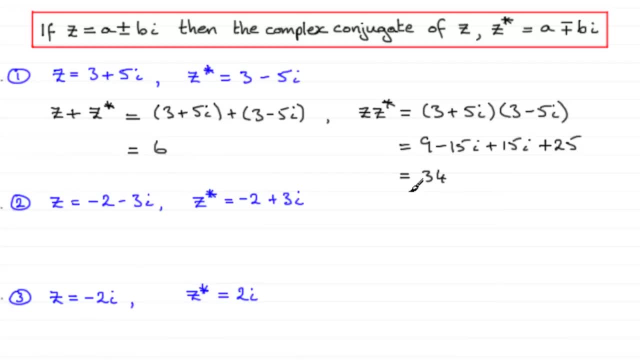 you get a real number again. You might like to just try these two just as a short exercise. Check out that if you add these two together, you'll get a real number. You might like to just try these two just as a short exercise. Check out that if you add these two together, you'll get a real number.